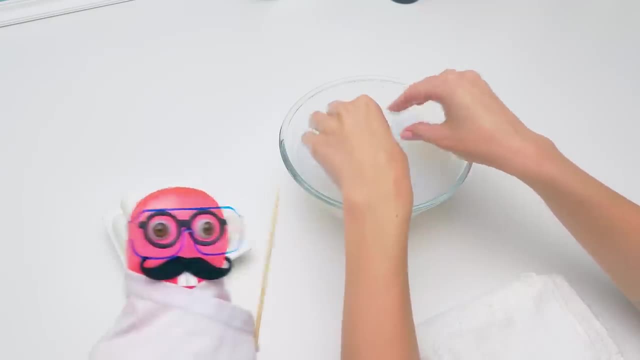 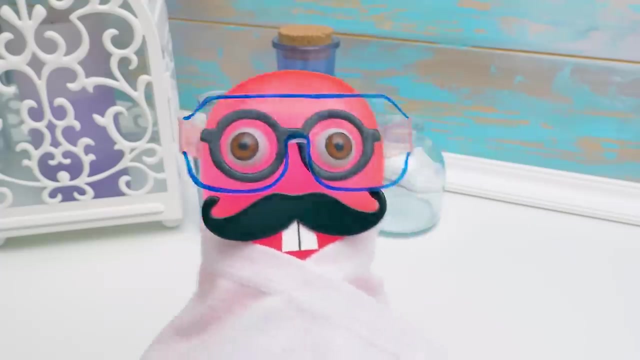 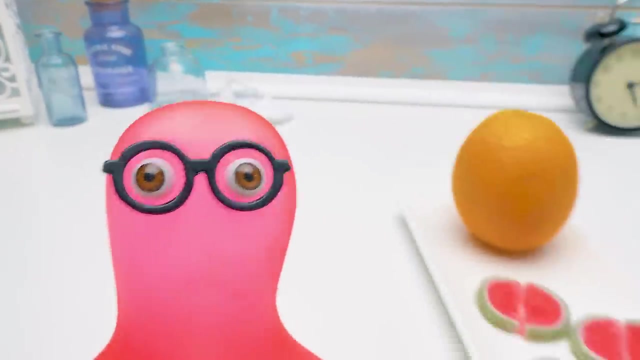 Professor, that was very interesting and informative. I am very happy to hear that Guys give a thumbs up if you think it was interesting And now we'll turn into. Now we'll turn into masters of soap making and create a couple of tasty masterpieces. 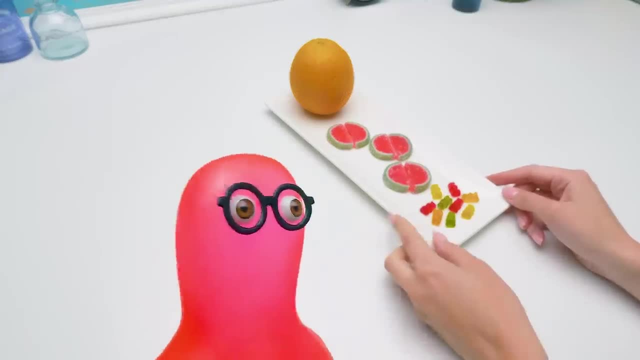 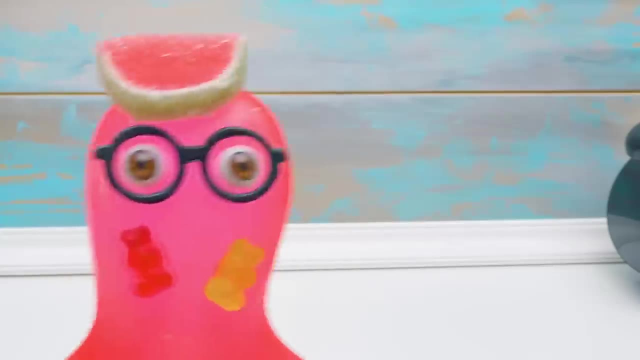 And I have everything ready here. What The ideas for the soap? of course, Oh, but you forgot one. While I'm preparing everything, tell us about your ideas, But it is obvious: Gummy bears, a watermelon and an orange. 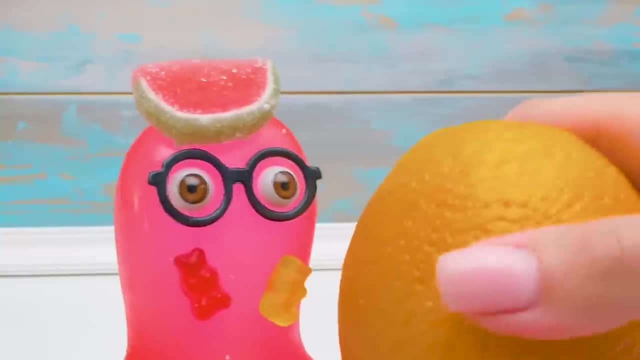 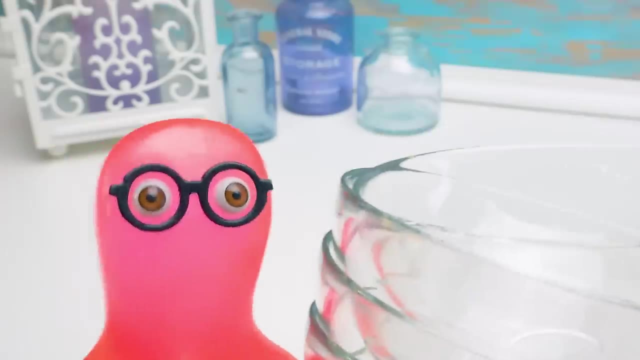 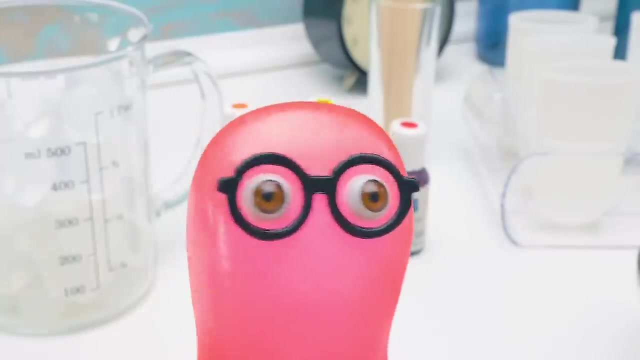 Well, the orange is more like your business. Oh, yes, I love fruit Guys. comment below: What kinds of treats do you like the most? So sue, all the ingredients for our task today are ready. Tell us, what will the first soap be made out of? 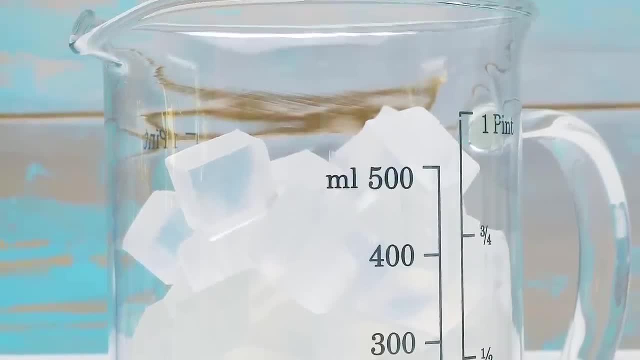 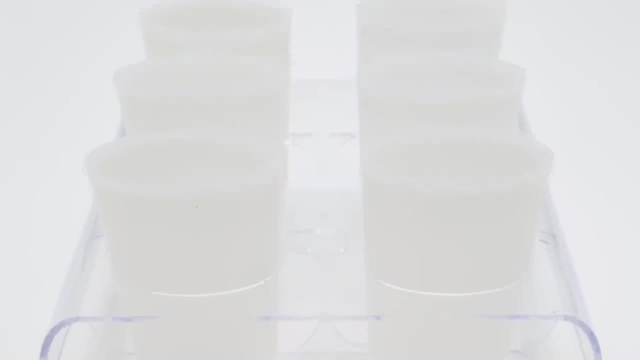 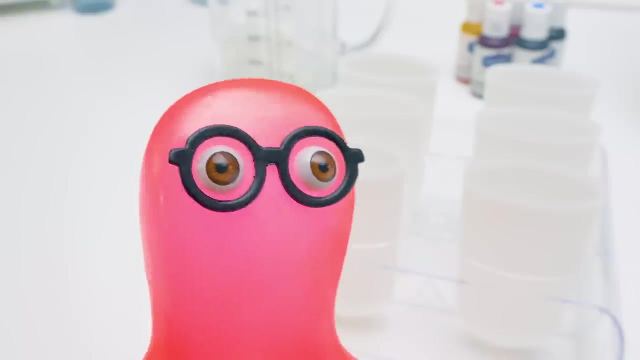 First we'll need soap base, Then five bowls, six sticks, a spoon, a special popsicle mold and five colors of soap coloring. A popsicle mold- Oh, it'll be a popsicle soap, Yay. So, guys, are we ready to start? 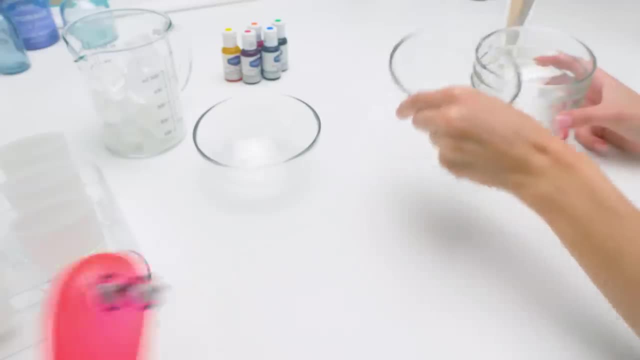 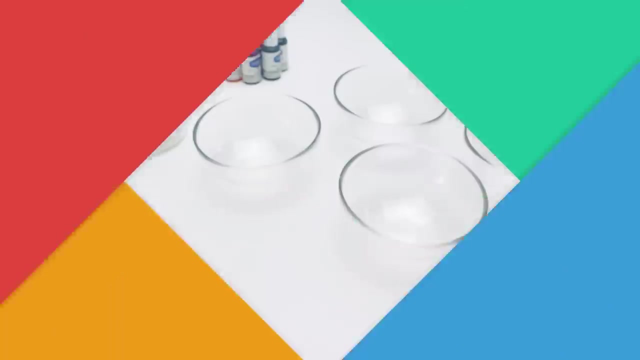 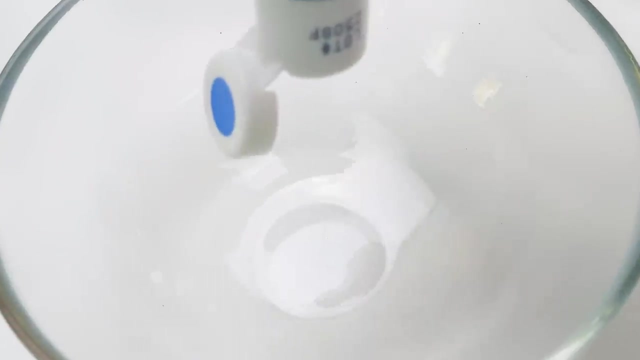 Let's start with the first soap. Here we go, Wait, wait, I don't think everyone there is subscribed to the channel yet. Nope, Seeing things. Let's start. What will we start our soap craft with? First, we need to take soap coloring and pour each of the colors into the bowls. 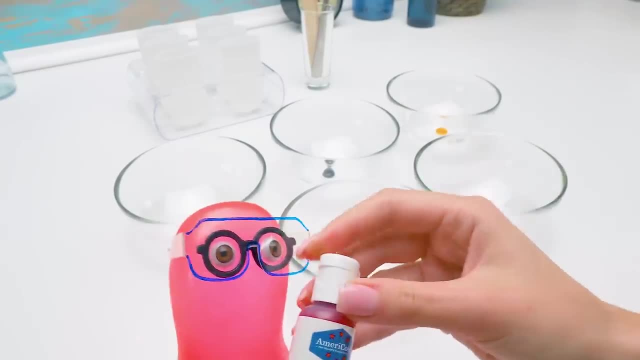 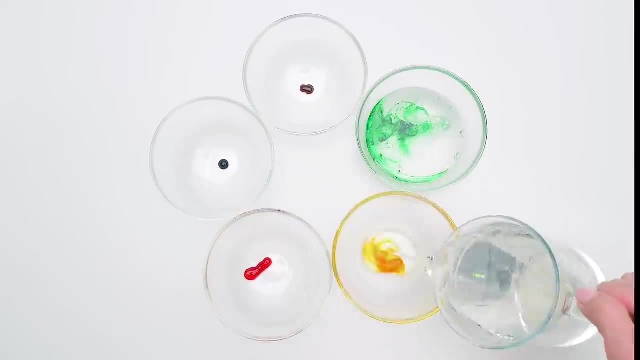 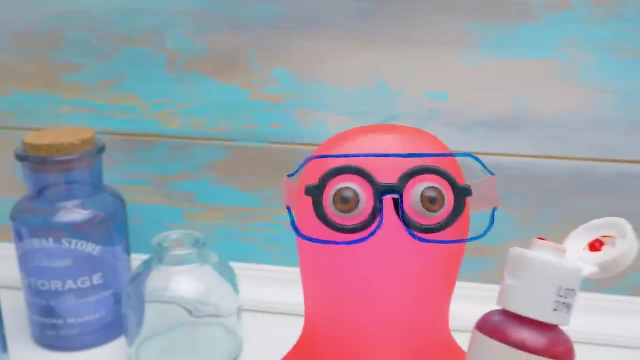 Oh, Sue, can I help you? Sure, Take the orange one. So done, You're a real pro. Now we're adding the soap base which we melted in the microwave earlier. Oh yeah, I am a pro, A very modest one, But you can still give me a thumbs up, considering that I brought you a spoon to pour the soap with. 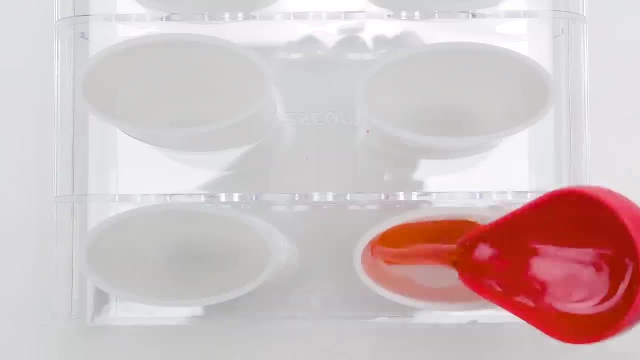 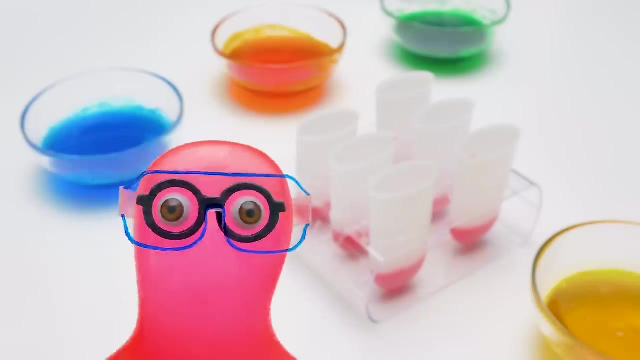 Oh, thank you, Sammy. Let's proceed Now. we take the spoon and, for example, the bowl with the red soap and pour the soap carefully into each special mold. And now let's add some yellow soap- Great idea. And then we also place a stick into each mold. 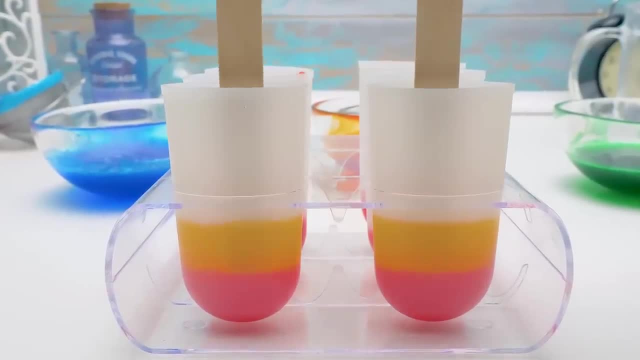 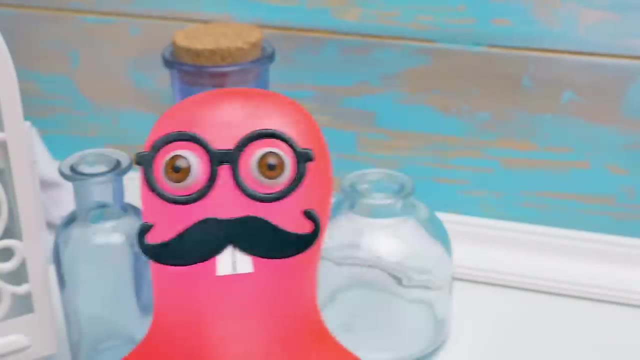 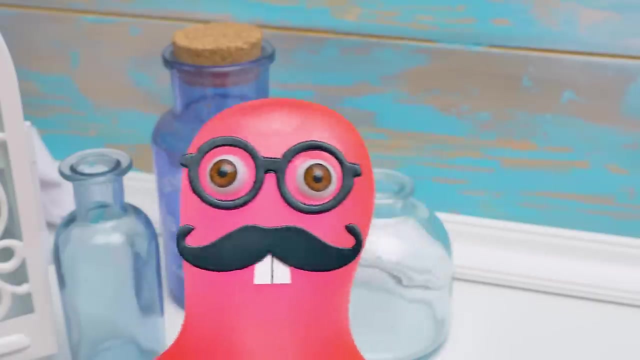 Like this, Sue. it's time to add the rest of the colors. And meanwhile, here is another soapy fact for you. The very first time soap was mentioned was in the year 2800 BC. It is incredibly ancient: Done and done. You only need to wait a little. 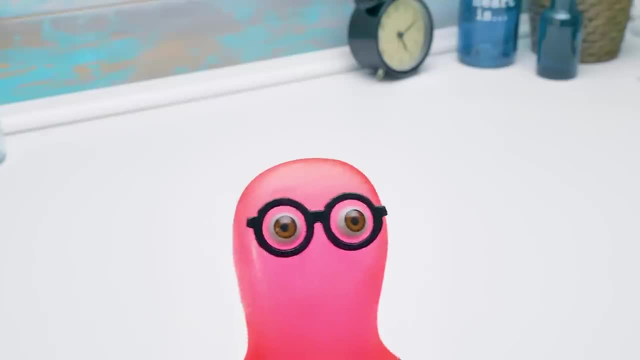 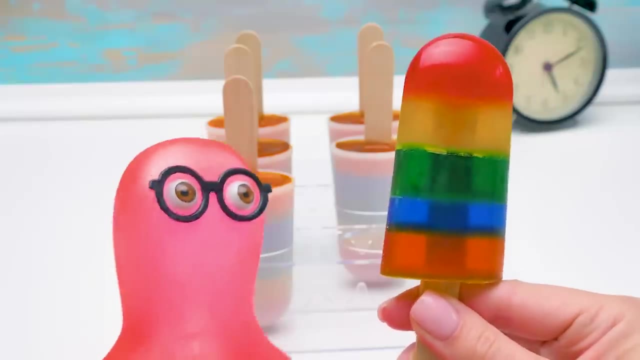 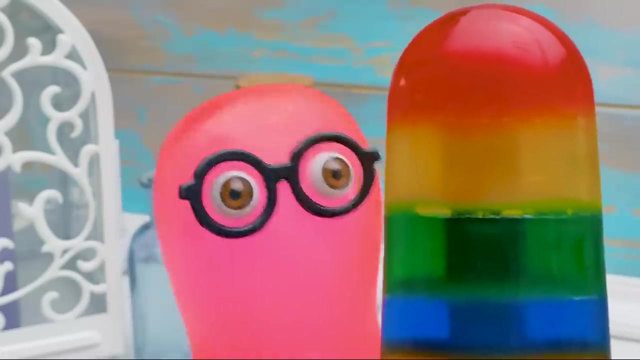 Wow, I can't wait to see our pretty popsicles. Wow, Voila, Ta-da, And it will really soap up. I can't believe that it is just just soap and not a real popsicle. We can test it in the bathroom when we finish all types of soaps. 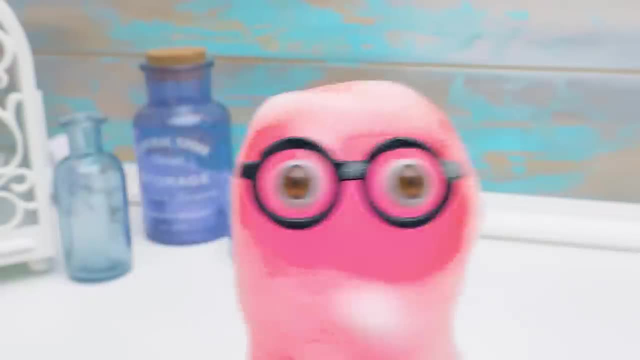 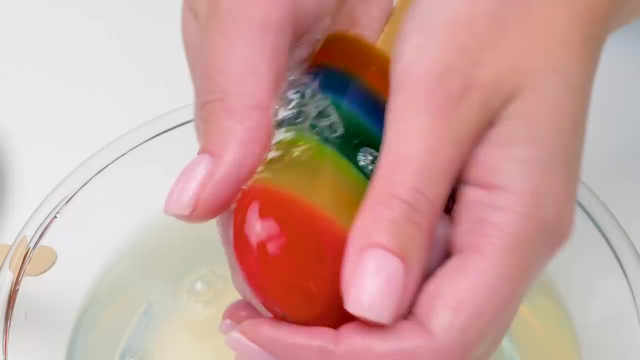 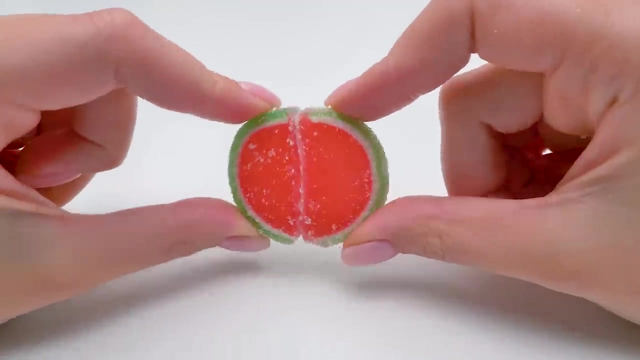 No, Sue, this is unbearable. Why wait when we can try it now? Okay, Sammy, you win. Mmm, my favorite Watermelon. Now it's your turn. When I smell a watermelon, I always think of summer. 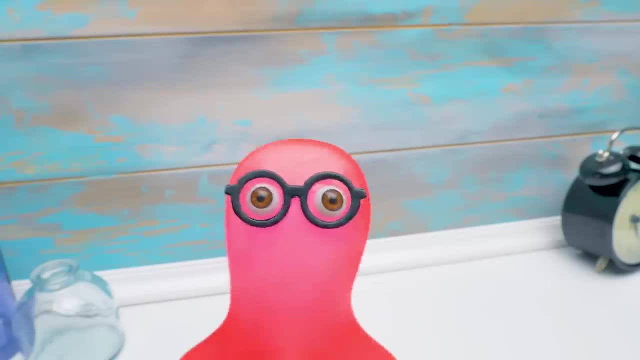 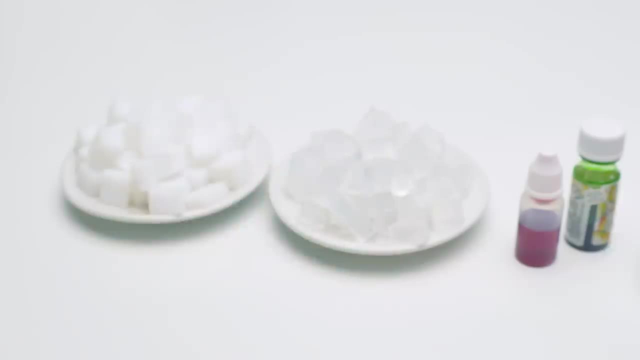 Write in the comments if it's the same with you. So, Sammy, can you tell us what we need for the second craft? Well, we'll need watermelon scent, White soap base, transparent soap base, red and green coloring, black soap pieces, molds. 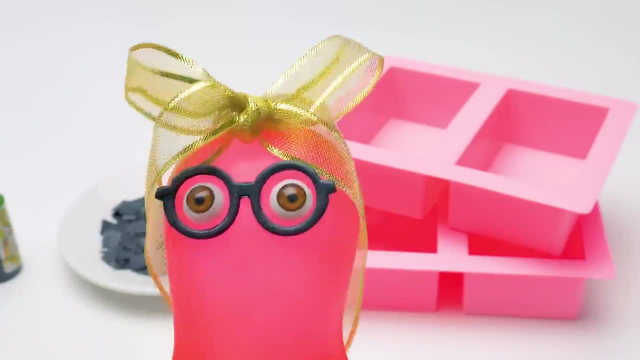 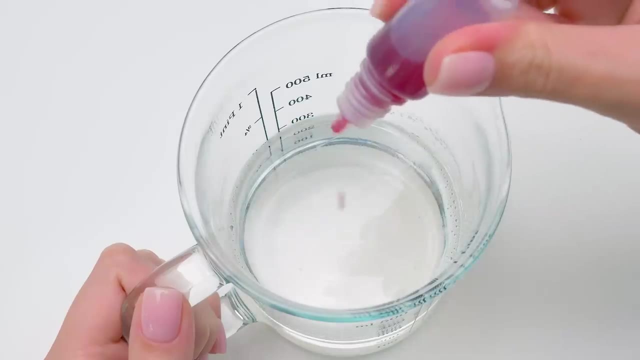 Plus something that I like very much: a ribbon for decor. Then let's create: We'll add our watermelon scent to the microwaved melted soap base, Then the red coloring And mix them well. Can I explain what's next? 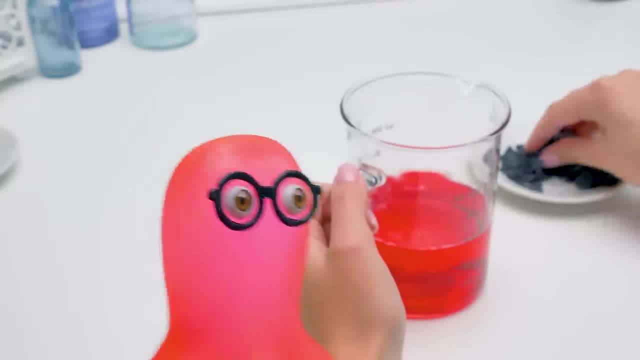 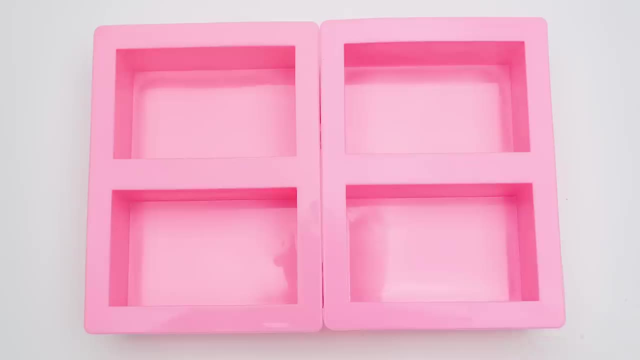 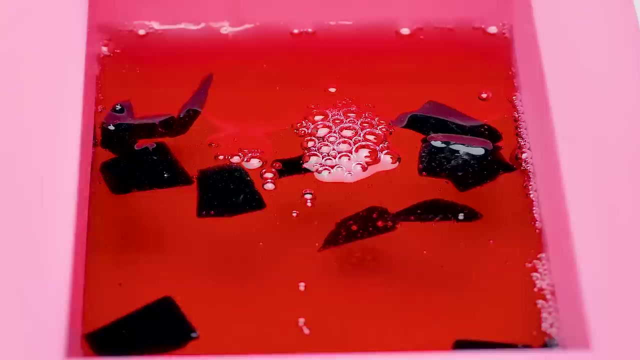 Go ahead, Considering that this is watermelon pulp. here we add Seeds- Hey, I'm talking here Right- seeds made of black soap pieces, And now we pour everything into the mold. Don't spill a drop Sue. The red soap should harden, and then we add the white soap. 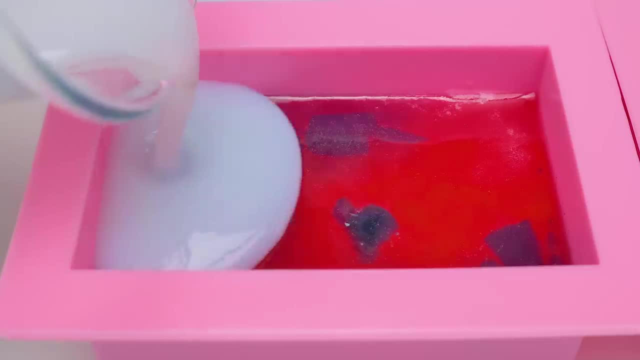 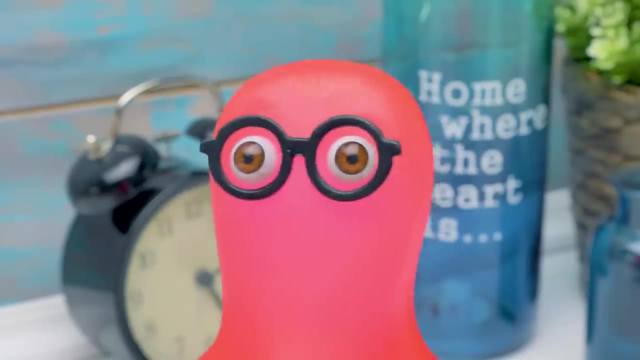 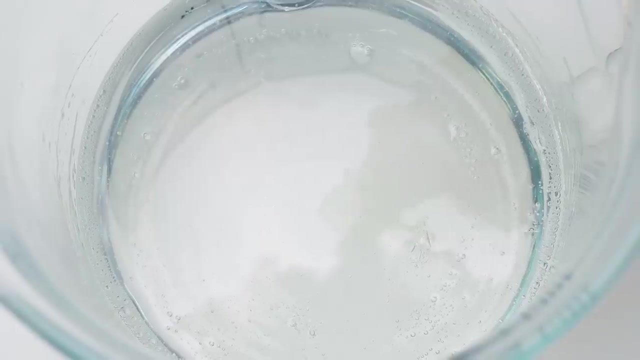 And we wait again. Susie, what do you know about soap gilts? Well, I know that they appeared in the 7th century AD, But when the factories came, all the gilts disappeared, since it became so easy to produce soap. 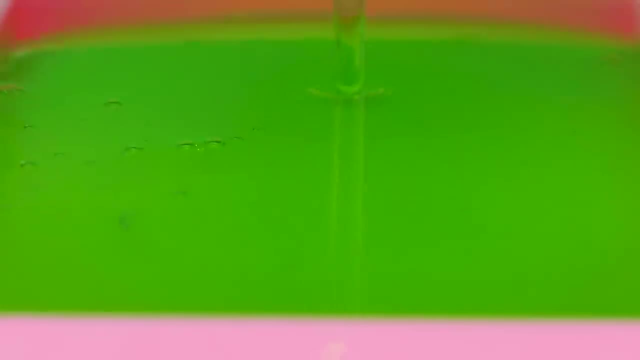 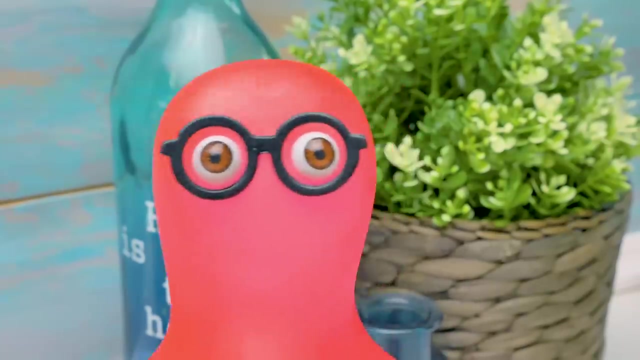 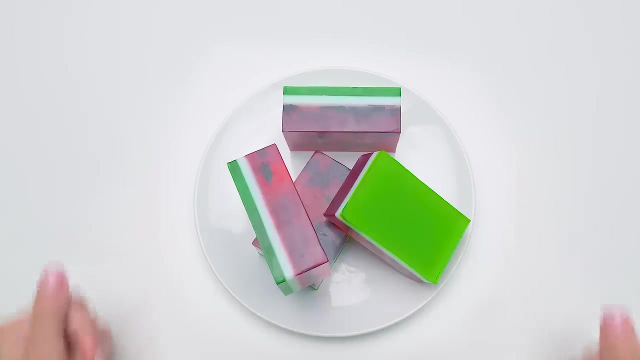 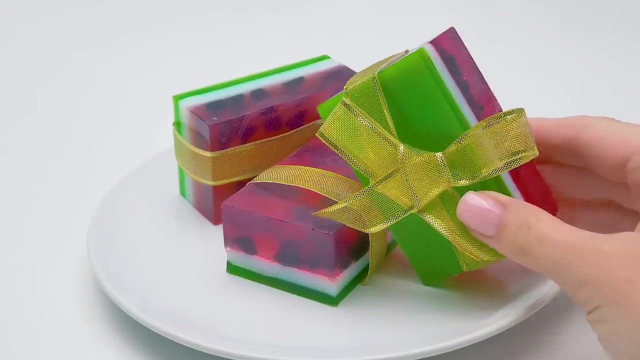 Attention. Here comes the green. What a bright color. Hmm, I am sure our gilts won't fall apart And our soap needs to set again. Let's take out our soap, Hop And hop And decorate it So beautiful. 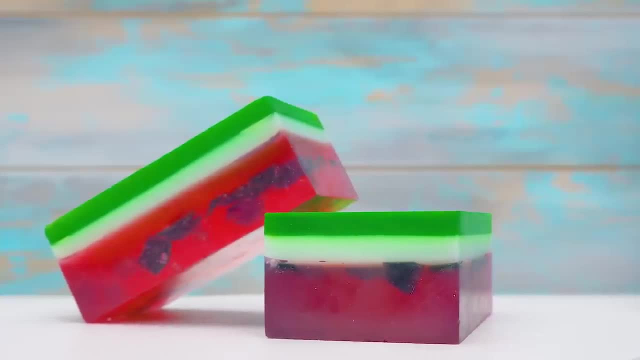 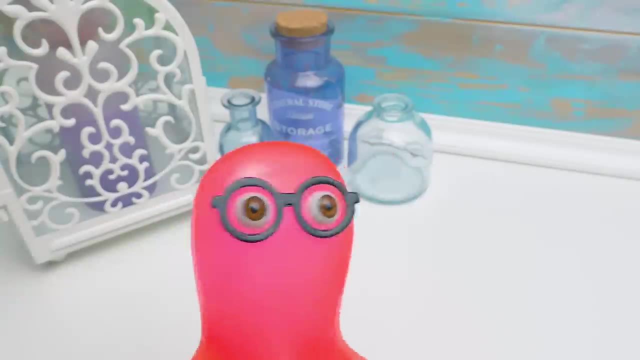 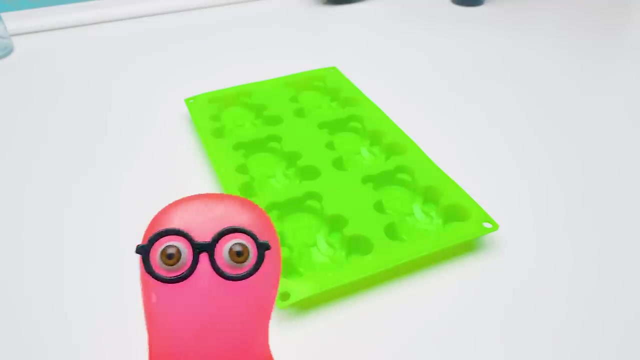 Yeah, I guess those who don't like to wash their hands after playing outside will definitely change their minds after they see such awesomeness. I am so looking forward to the gummy bears. When will we make them? Right now, Hooray And the soap will be as jelly-like as the real gummies. 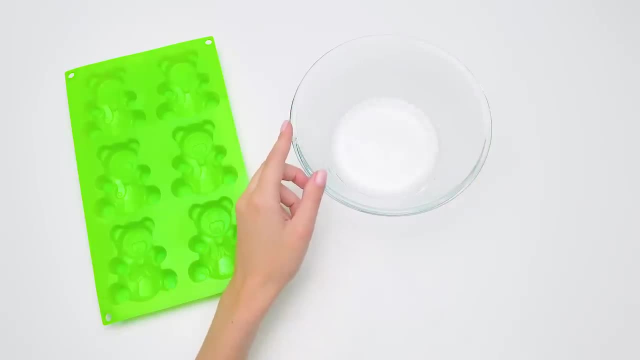 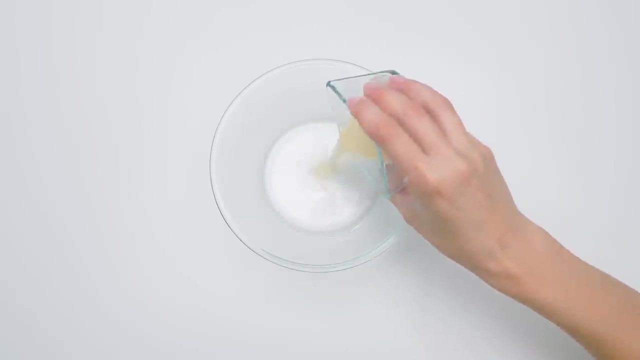 Of course, That's the best thing about it. Let me show you everything. I'm ready to listen, since I want to become the best member of our guild. Good, Listen then. First, we'll add some gelatin into our bowl. 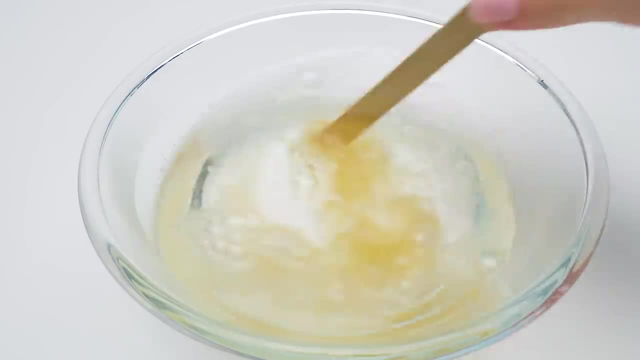 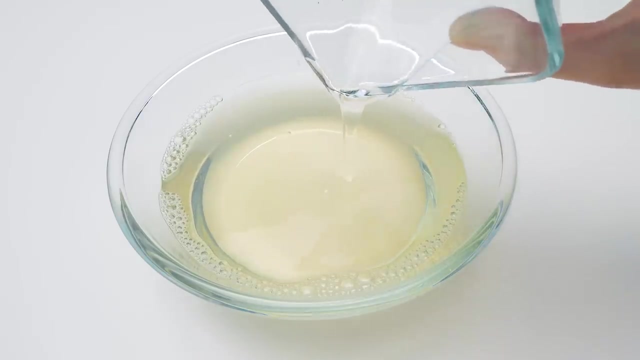 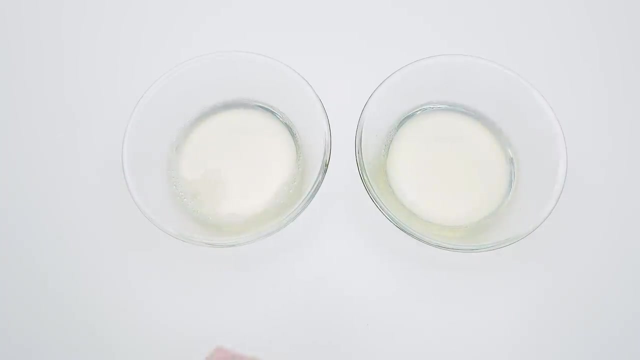 Then we need to pour really hot water. Be careful with that. Now we stir it until the gelatin completely dissolves. Next step is the liquid hand soap. There we go. I poured the mixture into two bowls. If you make your soap in just one color, there won't be any need to separate it. 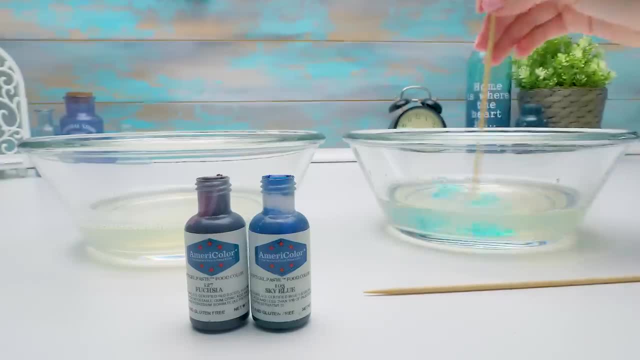 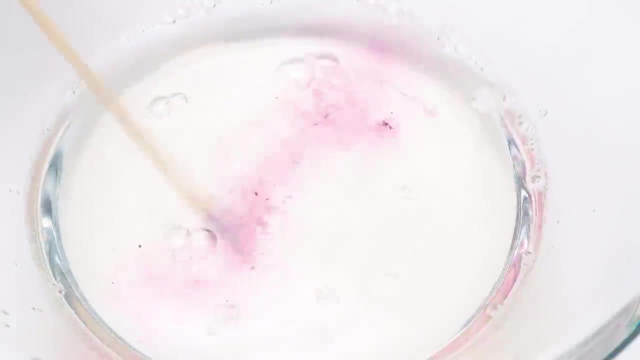 Then we'll add coloring into each bowl, Just like that. I am fond of colors. That's why I make two types of gummy bears. Now we pour our mixture into the molds. Actually, if you're not a fan of gummy bears like Sam, you can use any other molds, like hearts or stars, for example. 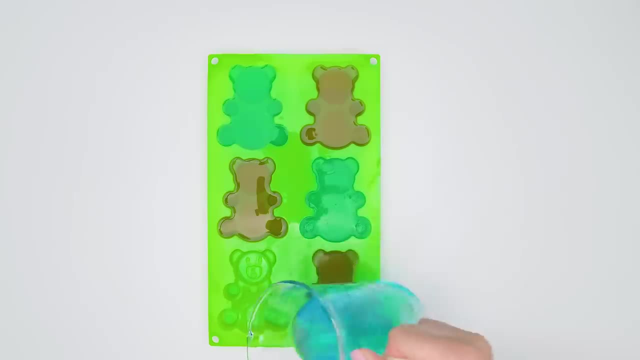 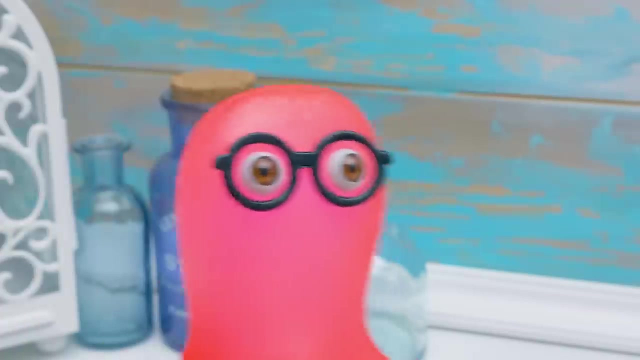 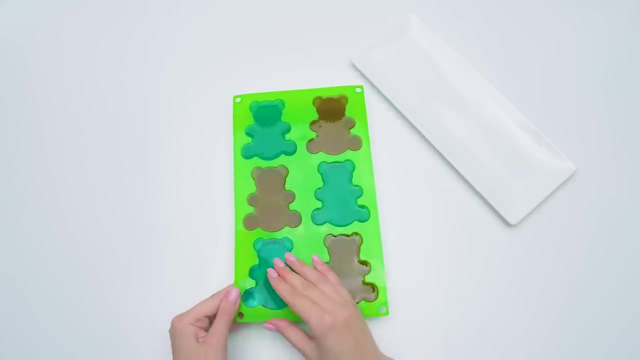 It's up to your imagination. Next, we let it chill, I'll be right back. Guys, do you like experiments? Let's test our soup, Sammy. our bears are ready. Sammy, where are you? You wanted to see them so much. 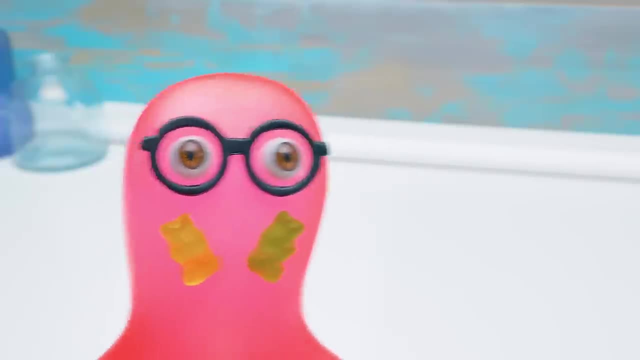 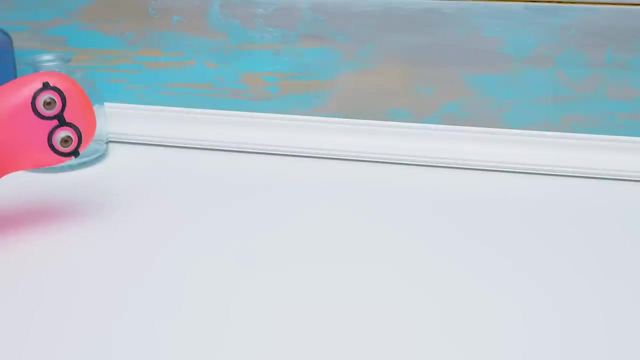 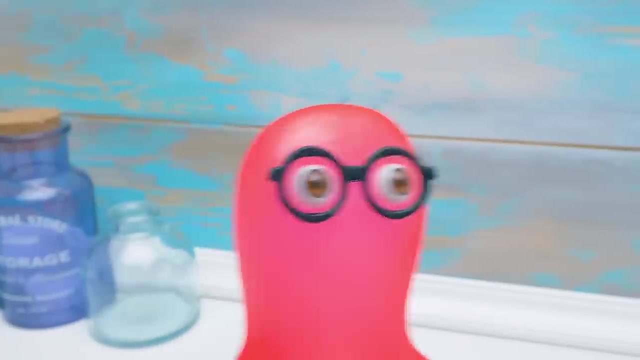 Sammy, We'll check to see if Sue can tell an edible bear from a soapy one. We'll leave them here and watch from our cover. Aha, here you are. You shared such a tasty treat with me, Thank you. You can't be fooled that easily. 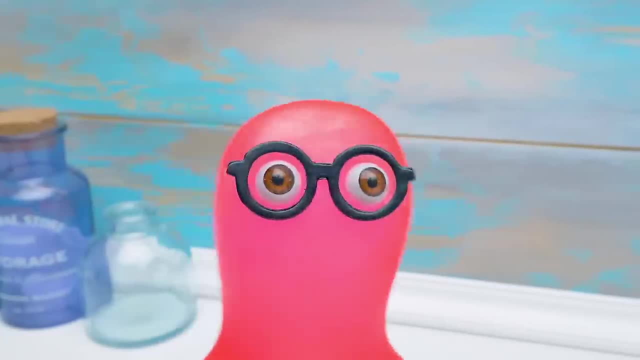 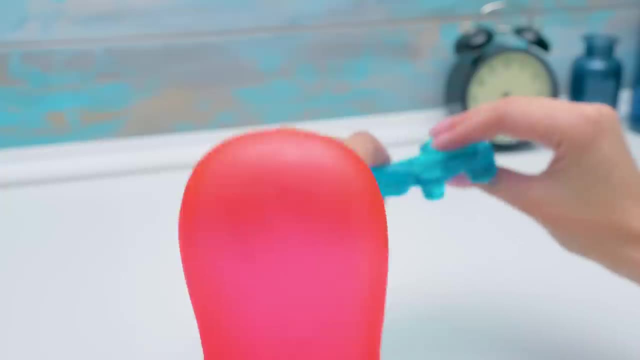 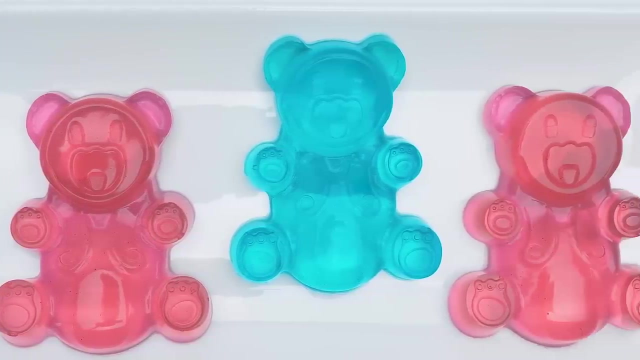 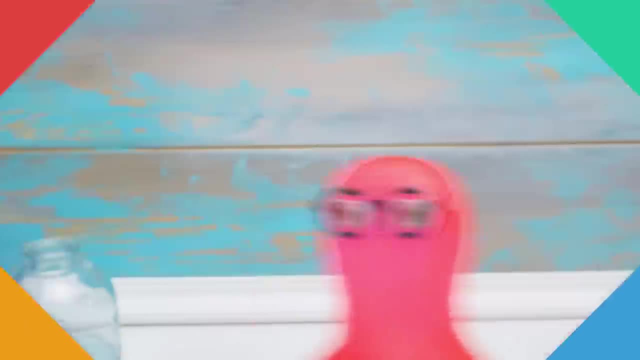 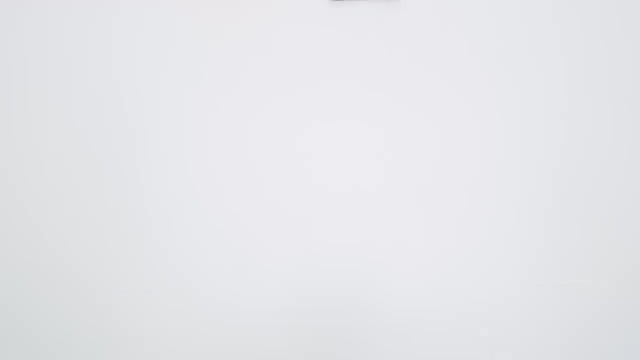 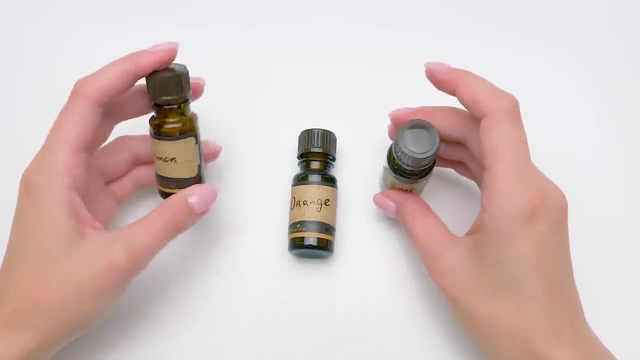 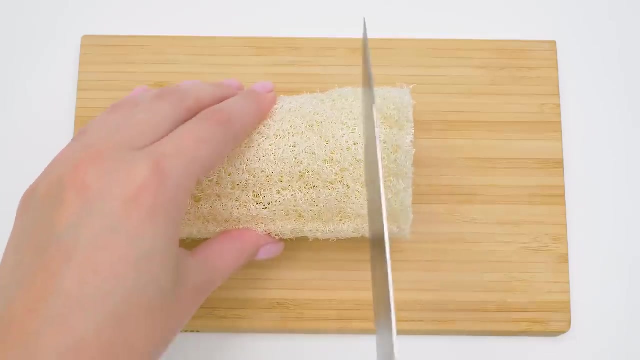 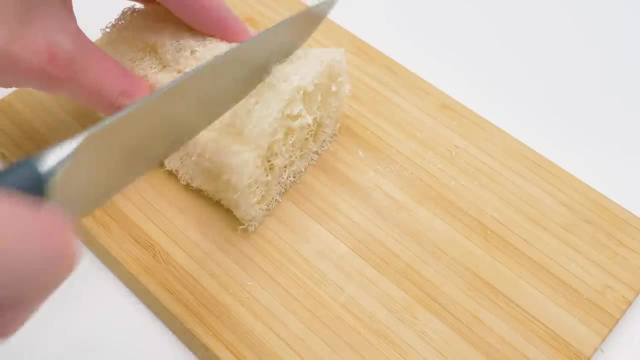 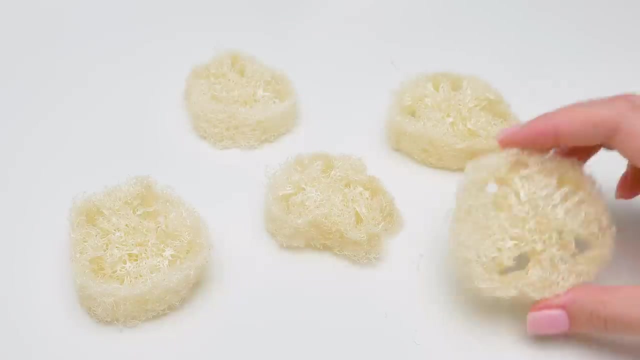 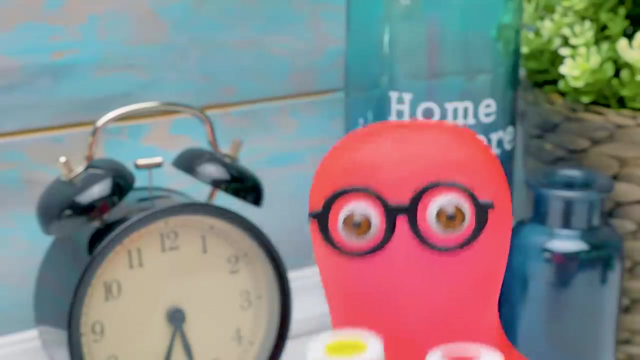 Awesome, Awesome, Awesome, Awesome, Awesome, Awesome. Oh, it reminds me of citrus, Correct, We, as Soap Guild members, need to be very creative, Sue. since you're making citruses, I brought you three different colors. Oh, that's great, Sammy. 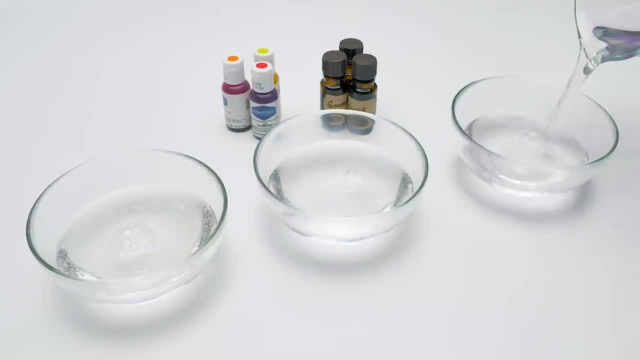 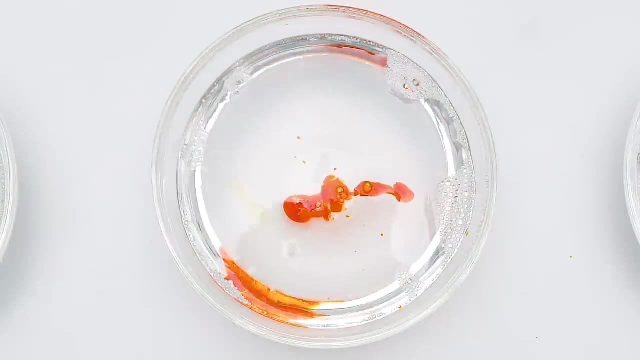 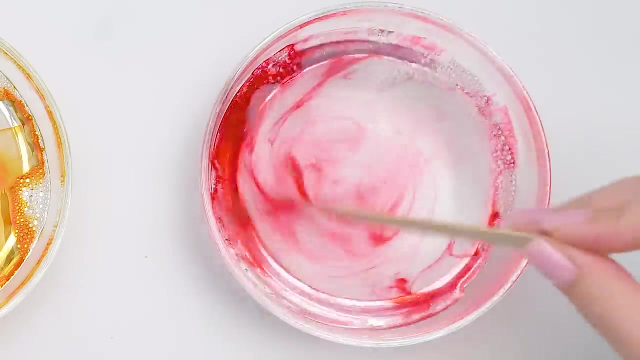 You're becoming a master of the soap craft. So in this bowl we'll add lemon oil and yellow coloring, Into the next one, orange oil and orange coloring, The last one grapefruit oil and red coloring. Now we mix everything really well and pour into the molds. 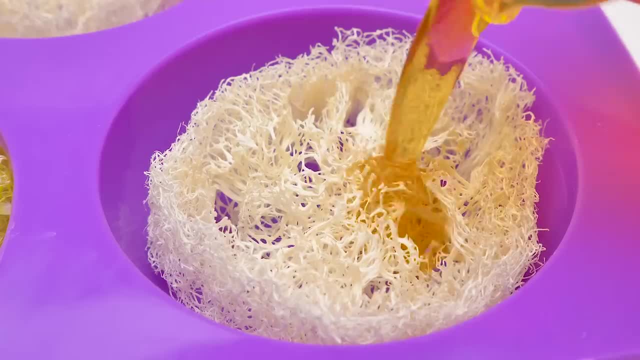 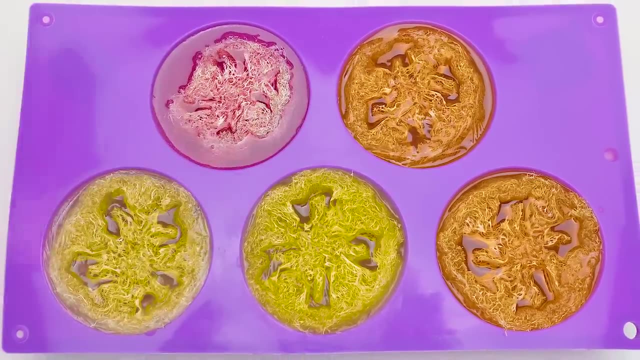 It's good that now the soap making process is so easy. In the past it was quite tough And the smell wasn't good at all. Everything changes, Sammy. OK, we'll leave our soap to set now. Good, good. 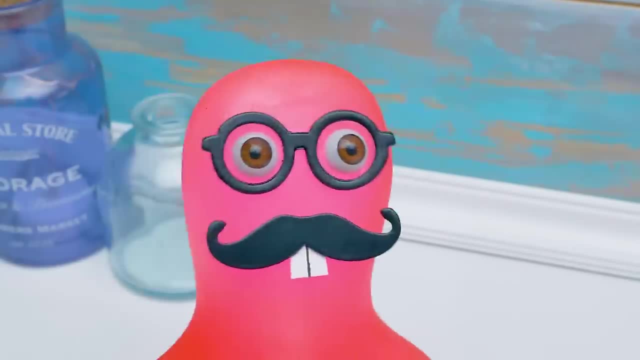 I want to tell our viewers one interesting fact. Did you know that soap needs to mature just like cheese? It's nice that you know that Soap is not cheese and smells good. Otherwise I would not bear another foul-smelling product in this world.